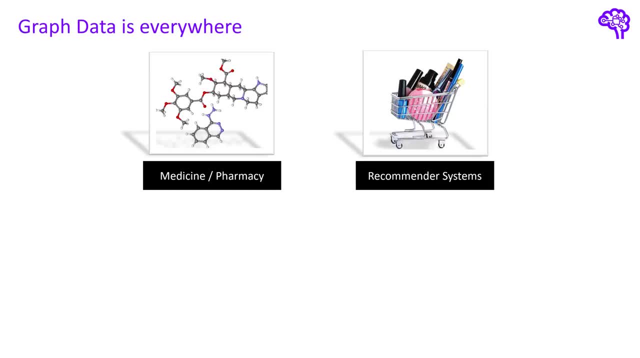 graphs to build useful recommender systems that suggest interesting products or movies. Another explaining example are social networks such as Facebook, where the people stand for nodes which are connected in certain relationships. The people can have features such as age, gender, favorite music and so on. Finally, you can also find graph structures in 3D games. 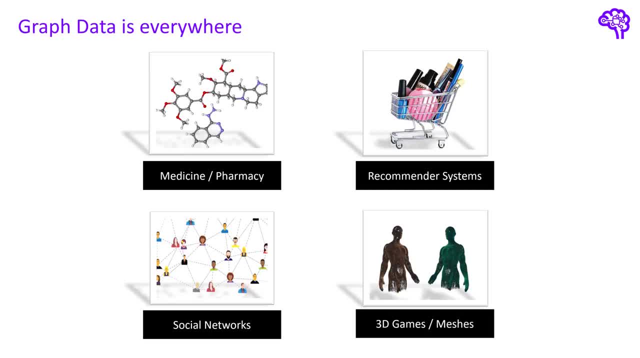 where the objects are usually modeled as a polygon mesh, which is a collection of vertices, edges and faces. These were just a few examples to give you an idea of how much graph data is available. But what can you do with this graph data in a machine learning sense? 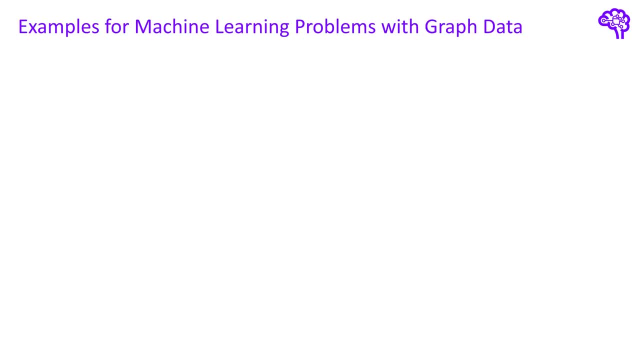 First of all, you can perform node-level predictions. This simply means that you have a graph with unlabeled nodes and want to predict attributes about these nodes or classify them. GNNs, as we will see in a second, will use the information of the other nodes in the graph. 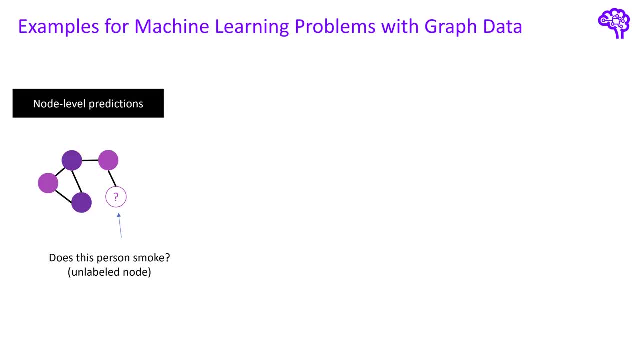 to infer on these unlabeled nodes. Another possibility is called link prediction or also edge-level prediction. Here you just predict whether there will be a connection between two nodes in a graph. For example, this is used by companies to predict which customer is likely to buy which product next. So basically the connection between people and items. 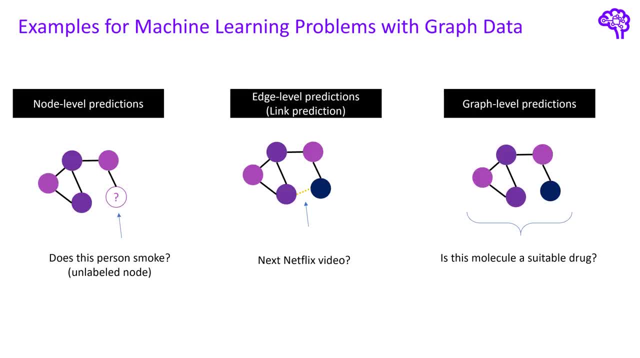 Finally, you can, of course, also use the whole graph as input and classify it or predict an attribute of interest. This is commonly done with molecule data, for instance, if you want to identify if a molecule is a suitable drug In the following. I assume that you are familiar with the 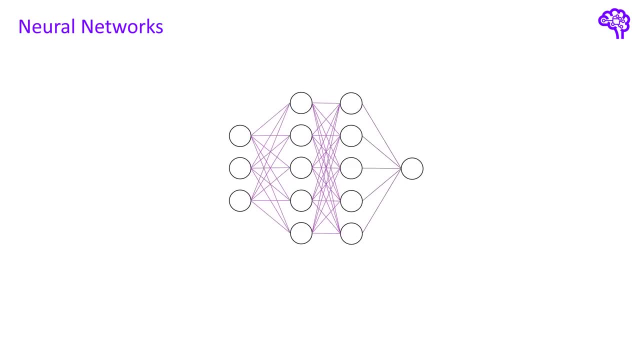 the inner workings of neural networks, as GNNs simply extend classical feedforward models. In the past, there were a variety of other approaches to handle graphs, such as hand-grafted features as input for machine learning models. However, graph data has some interesting properties that make it difficult to work with. 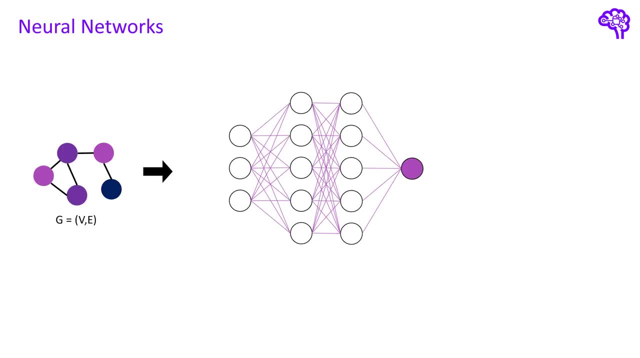 In a second we will find out how GNNs cope with all of these difficulties. As you might know, neural networks typically expect a fixed size input. This brings us to the first difficulty of graph data. The size and shape of a graph might change within a dataset. 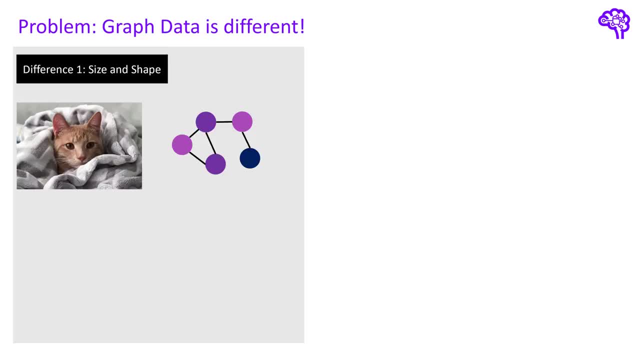 This might also be true for other data types, such as images, but here you can simply resize, pad or crop the images to the same size. Such operations are not defined on graph data. If you have additional nodes or edges, you cannot simply remove them. 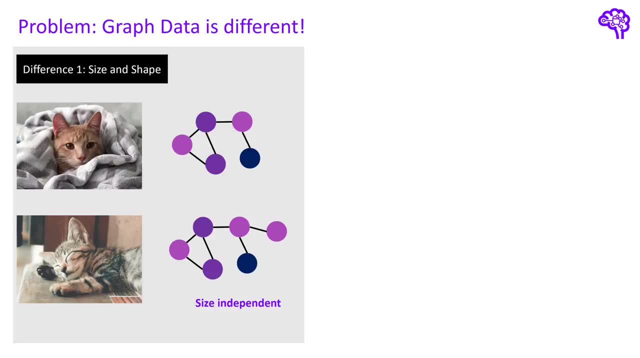 Therefore, we need a method that can handle arbitrary input shapes. Another feature of graphs, which is called isomorphism in graph theory, says that two graphs that look different can still be structurally identical. If you flip the image on the left, you get an entirely new image. 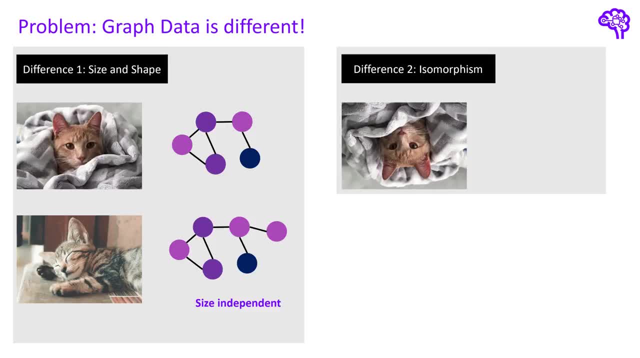 If you flip the graph on the left, however, the only thing that changes is the order of the nodes. The algorithm that is supposed to handle graph data therefore needs to be permutation invariant. This is actually also the reason why you cannot directly use the adjacency matrix as input. 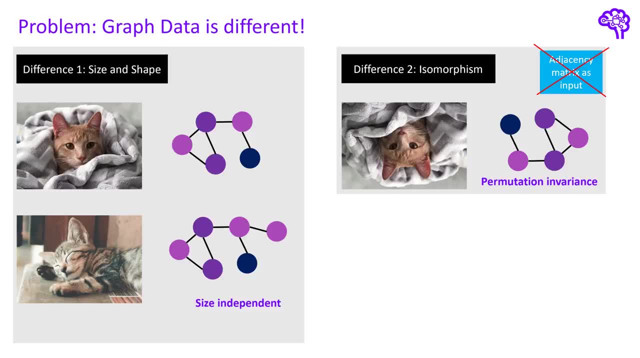 for the feedforward network, As it is sensitive to changes in the node order. Finally, the structure of graphs is non-Euclidean. For images, you have a clear grid that can be expressed by x and y coordinates. Graphs are dynamic structures that might lay differently in the space and distance metrics. 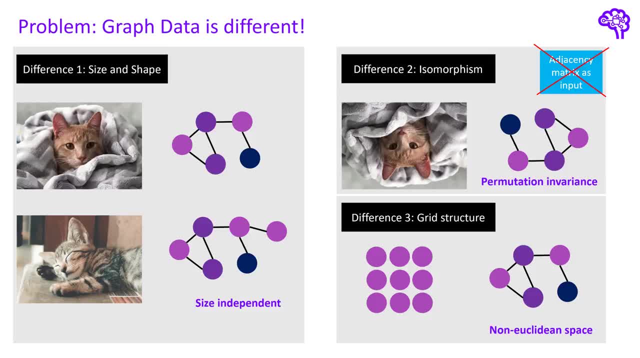 such as the Euclidean distance are not clearly defined. For instance, you cannot really say how close node A and B are. Of course, you can add 3D coordinates, But they do not incorporate the grid. This is also the reason why the machine learning area around graphs is called geometric deep. 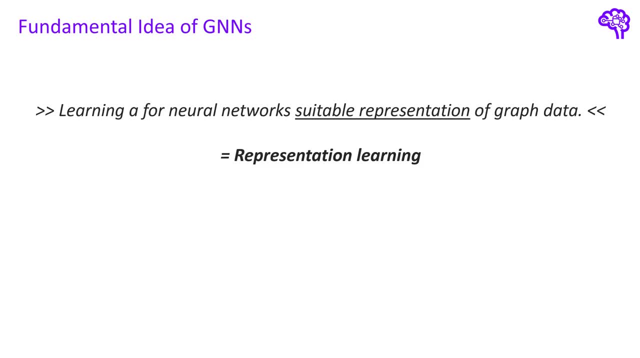 learning. The fundamental idea of GNNs is to learn a for neural networks suitable representation of graph data. This is also called representation learning. Using all the information about the graph, including the node features and the connections, stored in an adjacency matrix, the GNN outputs new representations, which are also called 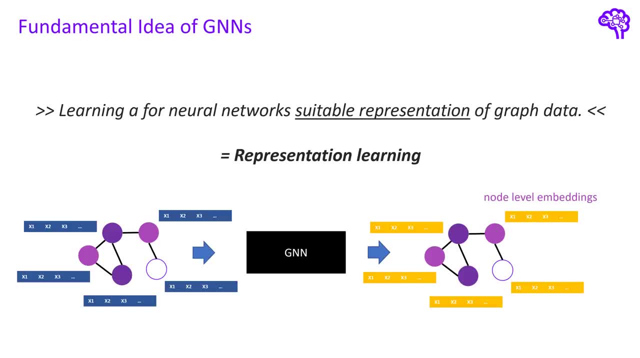 embeddings for each of the nodes. These node embeddings contain the structural as well as the feature information of the other nodes in the graph. This means each node knows something about the other nodes, the connection to these nodes and its context in the graph. The embeddings can finally be used to perform predictions. 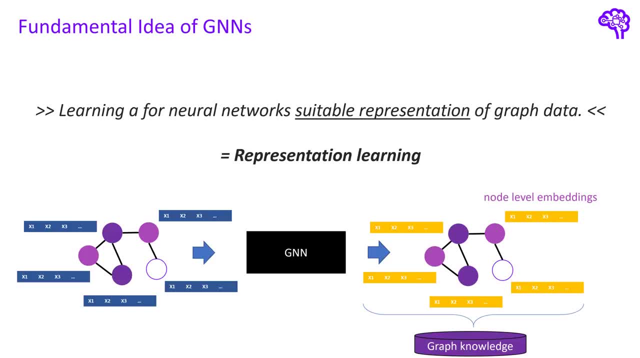 The way how you use them heavily depends on the machine learning problem you want to solve. For instance, if you want to perform node-level predictions, you would simply use the node embedding of a specific unlabeled node. For example, if you want to use a specific node embedding of a specific unlabeled node, you would simply use the node embedding of a specific unlabeled node.